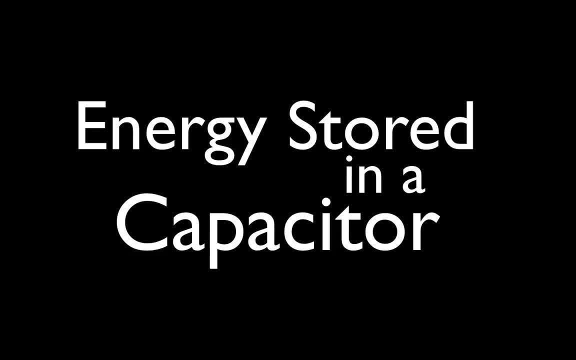 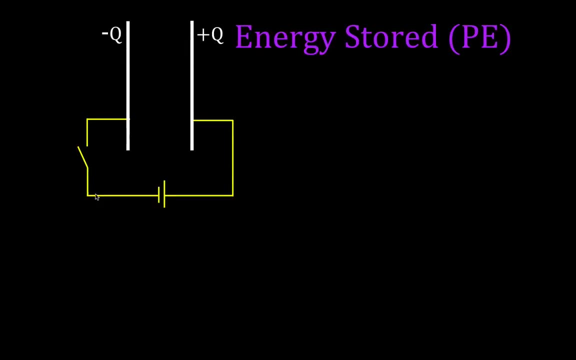 Okay, in today's video, as you can see, we are going to go over a discussion and talk about how to calculate how energy is stored and the amount of energy that is stored in a capacitor. All right now, this is a general diagram I have of a capacitor, And when we talk about energy, 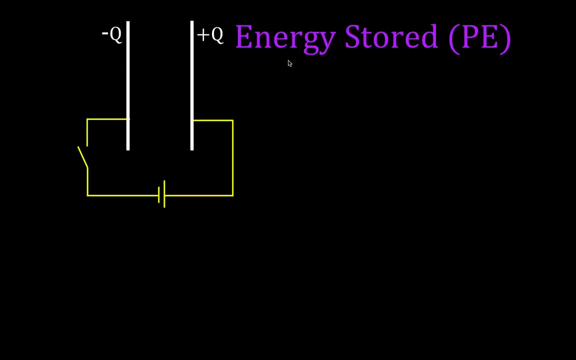 stored in a capacitor. usually you can say it two different ways. You can say that charge is stored, so capacitors store charge, but in order to store charge, the battery has to do work to move the charges from one plate to another. So really, when you're storing, charge the battery. 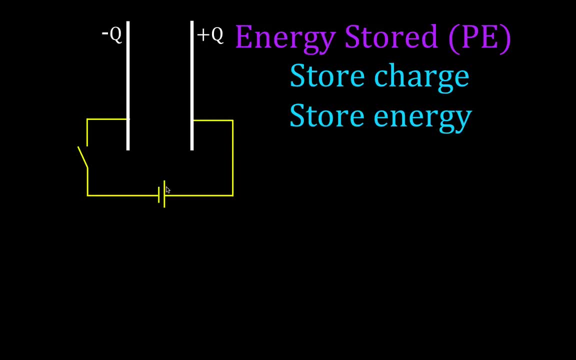 is doing work and therefore, what you're really storing is energy, and that energy can be released at a later time. Okay, so what we like to say is that the energy stored is equal to the work done by the battery to move the charges from one plate to another. 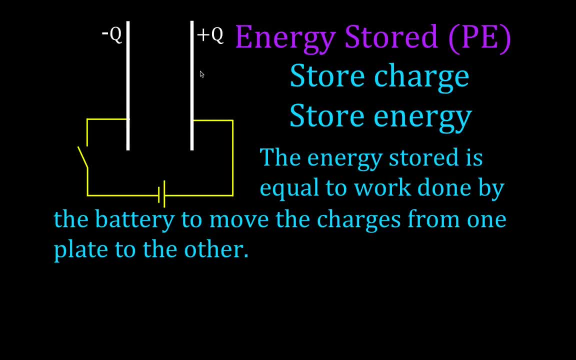 So what the battery does is it takes the charges, the electrons, the negative charges, moves them from one plate to the other plate. When it does that, it has to do work And, just like when you have gravitational potential energy, when you do work you store gravitational 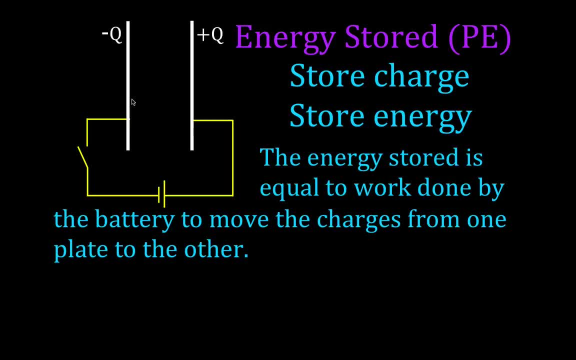 potential energy. But in this case we're not storing gravitational potential energy, we're storing electric potential energy. So the energy stored, the potential energy stored, is equal to the work done by the battery, And that energy, we like to say, is stored in the electric field between the plates. So when all of 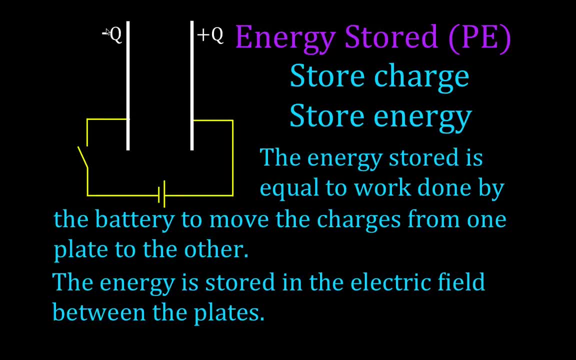 the charges have been moved over. we have a positive plate and a negative plate and we have an electric field that goes from the positive to the negative and the energy is stored in the electric field between those plates. Okay, so stored energy, stored charge, work potential. 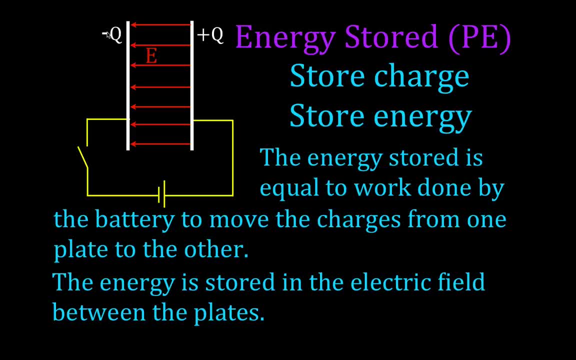 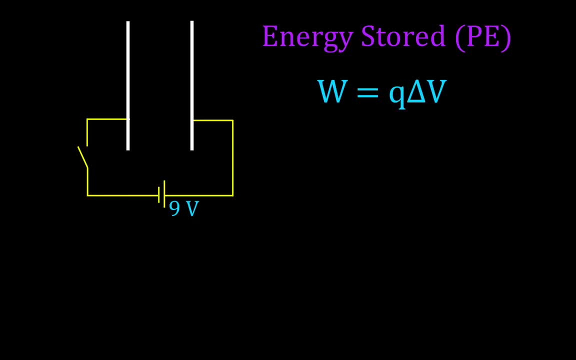 energy. the energy is stored in the electric field. Okay, now let's just look at a little bit more detail how we calculate that, how we calculate the work done, or really we talk about the amount of energy that's been stored, moving the charges. 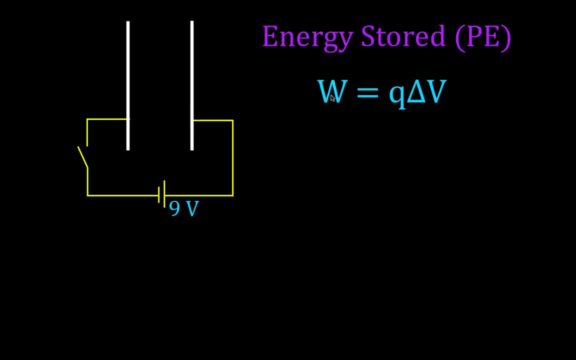 from one plate to another. Okay now, this is the equation that we used previously to calculate the amount of work it takes to move a charge through a certain potential difference. As I mentioned earlier, when you do work, you store energy. In this case, we're talking about electricity. 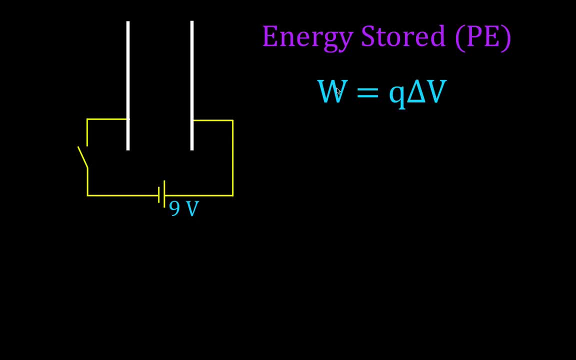 not electric potential energy. So in order to store that energy, the battery has to do work. or when the battery does work, it's going to store electric potential energy through the movement, okay, of those electrons. that's been moving a charge All right. now. what we're going to do, as you can see, 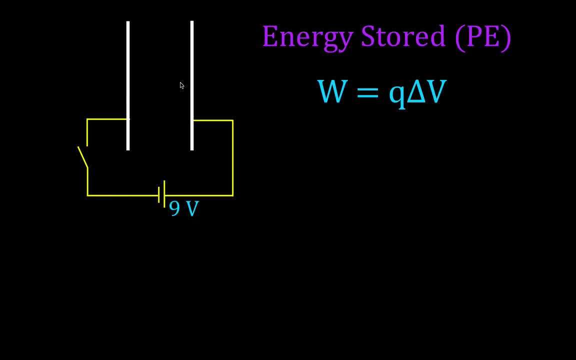 here. we have a nine volt battery, we have a switch and this is kind of a schematic of a capacitor. These are the parallel plates for the capacitor, and we're going to take one unit of charge, which is Q, and we're going to take one unit of charge, which is Q, and we're going to take 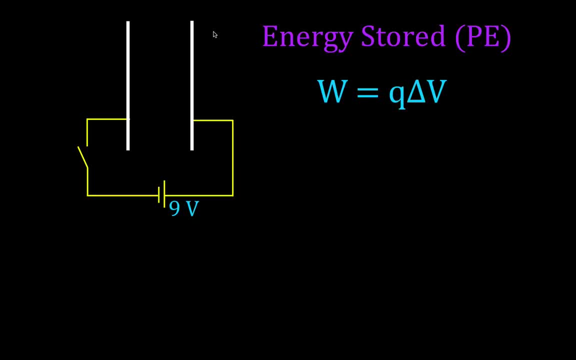 one unit of charge, which is the electron, and we're going to move that from one plate to another. Okay, so I close the switch and right when I close the switch, the charges start to move from one plate to another and we're going to kind of look at this one electron at a time. So the first 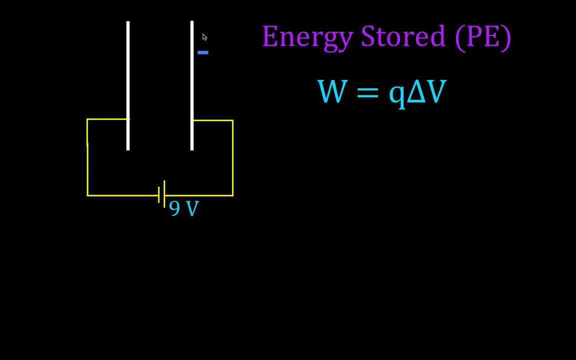 electron gets moved from one plate through the battery and to the other plate, And what we're going to do is now we're going to use this equation: the amount of work done is equal to Q, and the number of count drops the charge through the potential difference. 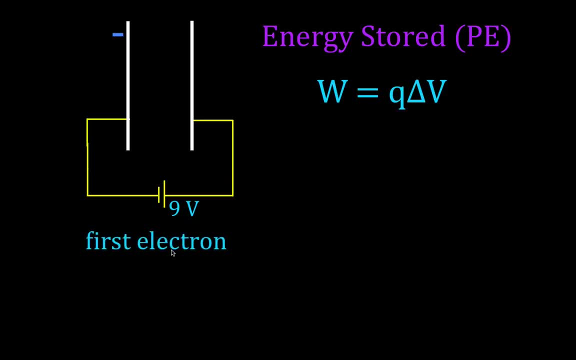 through which that charge is moved. Okay, I'm going to do that right down here for the first electron. Okay, the work is equal to the amount of charge. the charge on the electron is 1.6 times 10 to the minus 19 coulombs. 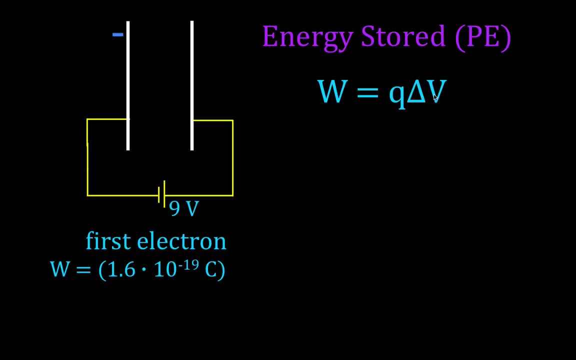 Now the question is in this case is what potential difference was that charge moved through? Well, you notice, we have a 9-volt battery and right when we close the switch, the charges start to move. But the very first electron 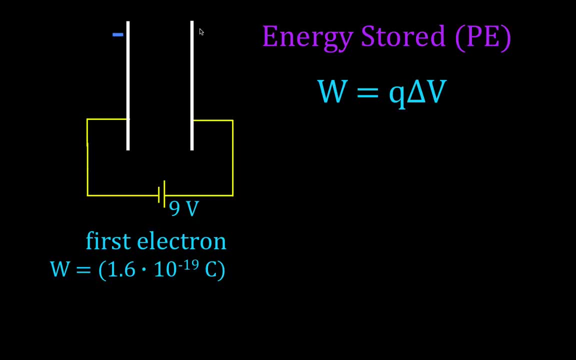 you think of it? electron per electron, the very first electron, when the very first electron is moved from one plate to the other, when it's moved- not before, but when it's moved- there is no potential difference between those plates. So we have charge, we have no potential difference. 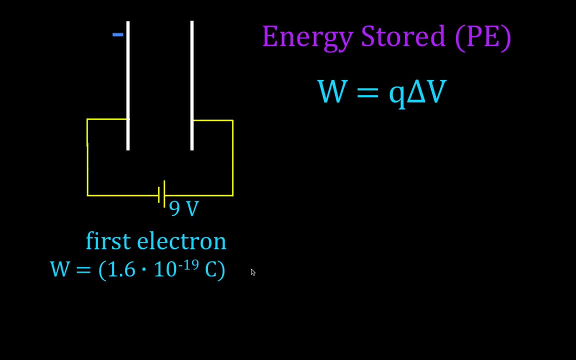 So down here it's work is equal to the charge times, the potential difference through which that charge was moved. Well, that charge was moved through no potential difference. So the work it takes to move the first electron is really zero joules of work. 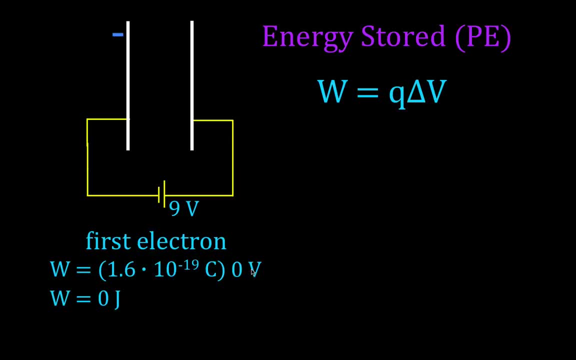 Zero joules of work is done to move the first electron. All right. Now the next thing we have, of course, now we have a positive plate and a negative plate And we're going to continue to do that: move the electrons over. 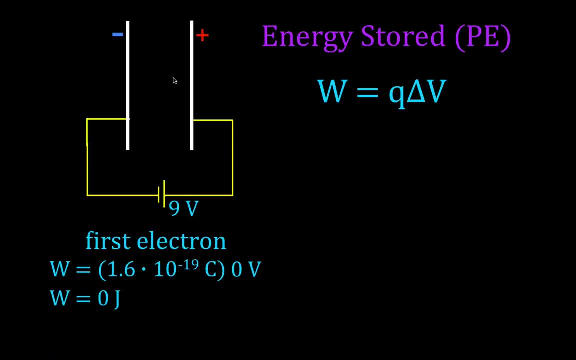 link of it, like kind of like moving them over one at a time. one at a time. That doesn't happen, one at a time, But you can kind of think of it like that until we have almost all of the electrons have been moved over. 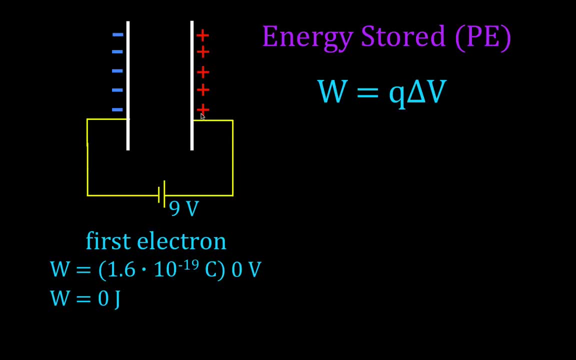 So we have: this plate is almost fully charged. This plate is almost fully charged, The capacitor is only full- almost fully charged. But we have one last electron that we need to move. The battery can move one more electron, So we're going to move that last electron over, like that. 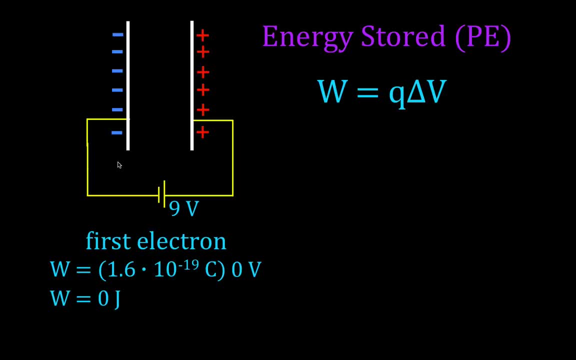 Now the plates are fully charged and no more electrons are moving from one side or from one plate to the other. Now let's calculate the amount of work it takes to move that very last electron using this same equation. Now we're doing this kind of electron by electron. 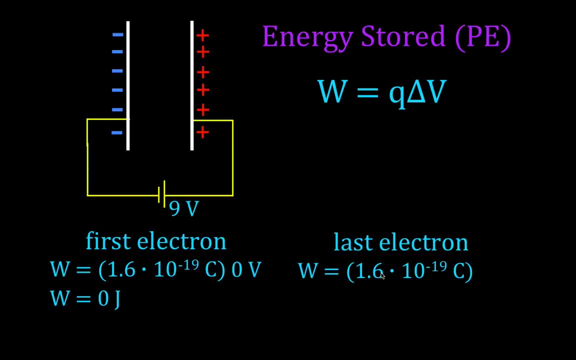 Okay, the amount of work is equal to the charge Q times the potential difference. What's the potential difference this time? Well, really, when we move the last electron, the capacitor is basically almost basically fully charged, So there's 9 volts across the capacitor. 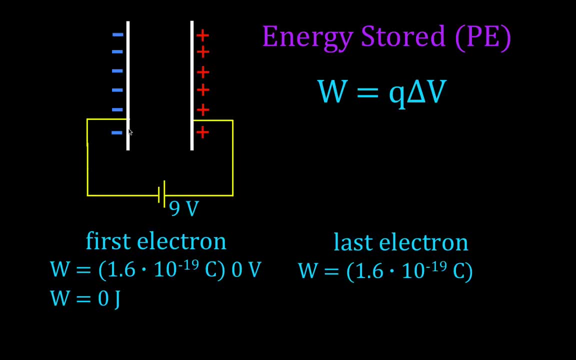 So that electron is moved through a potential difference of 9 volts. So we're now going to multiply that by 9.. 1.6 times 10 to the minus 19 times 9 volts is equal to 1.4 times 10. 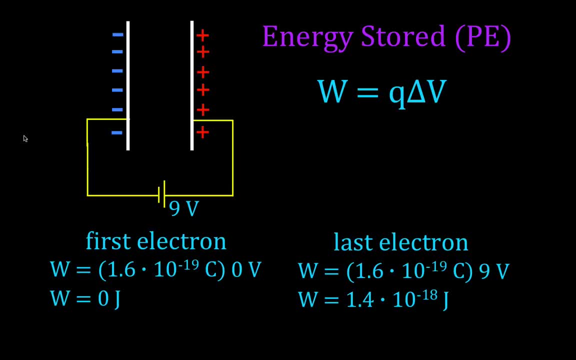 to the minus 19.. So that's the minus 18 joules of energy. Now, this over here is zero. That's the work it took, the energy that was stored to move the first electron. This is the energy or the work it took. 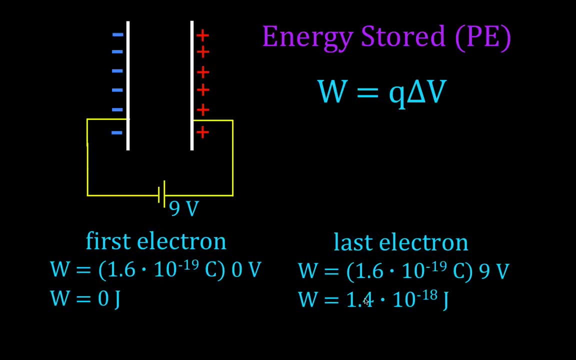 to move the last electron or the energy stored. Now what we could do is we could add all those up and sum them up, because the first one is zero, which we calculated, Then the next one moves through a little potential difference, So it's a little bit more than zero. 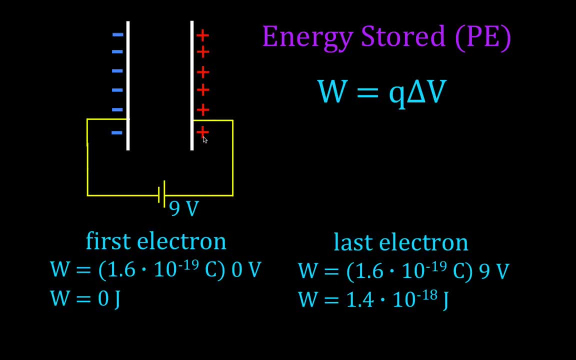 And then the next one is a little bit more and more and more and more, Until the last one. this is the work it takes to move the last one, And we can add them all up, But you could kind of see if we have the zero and the maximum amount. 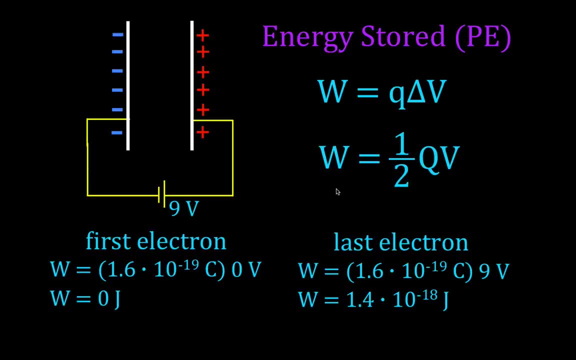 then the work is actually equal to one half the total amount of charge that's moved and the potential difference through which it's moved. Okay, So we can think of the whole amount of charge that's moved and it's moved through 9 volts. 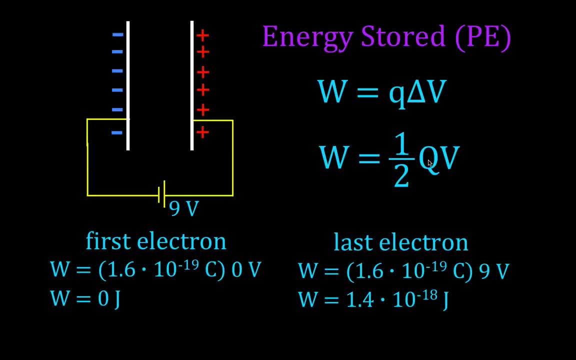 Okay, So now you can see we have Q, This is Q And this is Q. We change it from. this is usually written as a capital, Q, And this is the potential difference through which it's moved. So the work done, the energy stored, is equal. 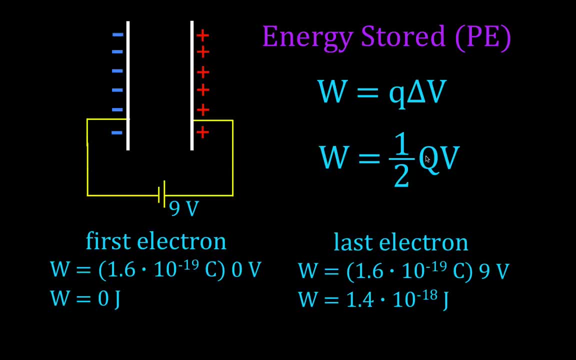 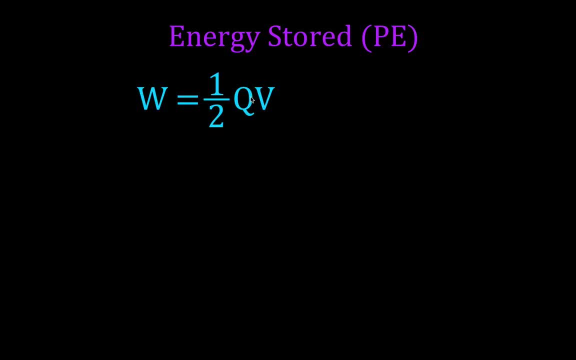 to one half times Q times V. All right, Now this is the same equation we had on the previous page. You often see this equation written three different ways, because this is W work is equal to one half Q times V The charge. 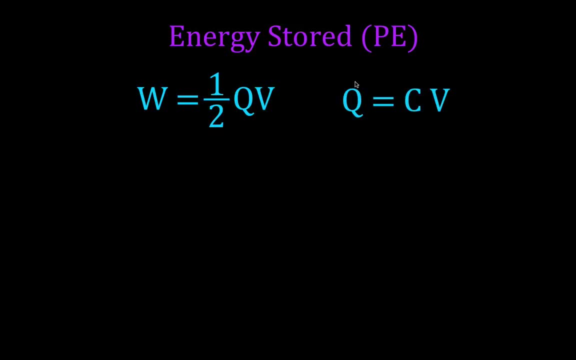 and the potential difference through which it's moved. But you remember, we had this equation which I like to call the capacitor equation: Q equals C times V And I can take this equation Q and substitute it in here for this Q. So I'm going to substitute CV, the capacitance. 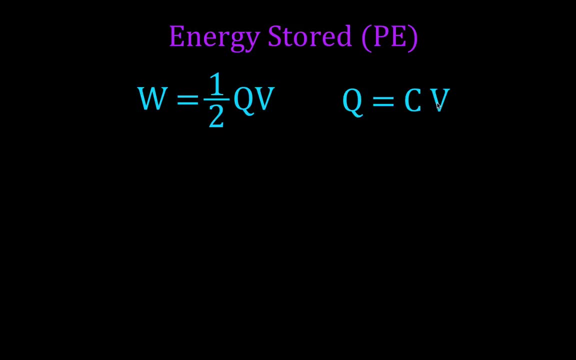 of the capacitor and the voltage across the capacitor. in here for this Q. And then I get that W, the work done or the energy stored is equal to one half C. This is this C, And I have an extra V, So it's V squared, the voltage squared. 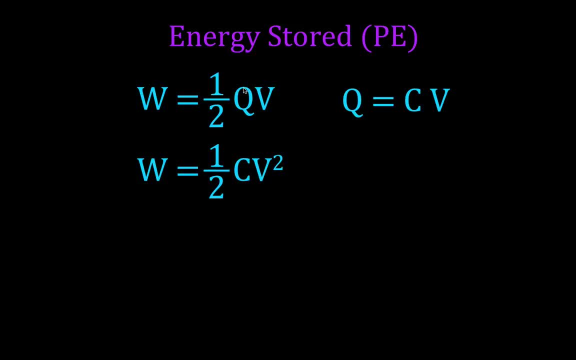 One half CV squared. Now I can also in this equation- I can rearrange this equation- solve it for the voltage. Okay, The voltage is equal to the charge divided by the capacitance. I can also substitute that in here And then you'll see we have Q squared over C. 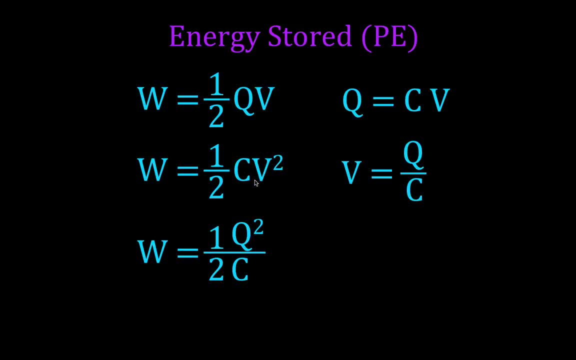 So this is another form of that same equation: The work, the energy stored, is equal to one half Q squared over C. Okay, So that's the three ways, the three different ways. you'll see this equation written once when you know the voltage and the charge, once we know the voltage.